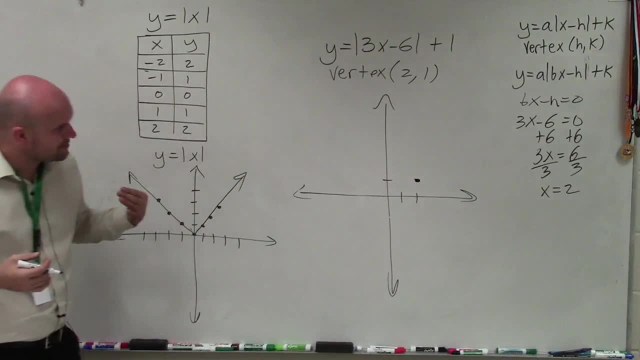 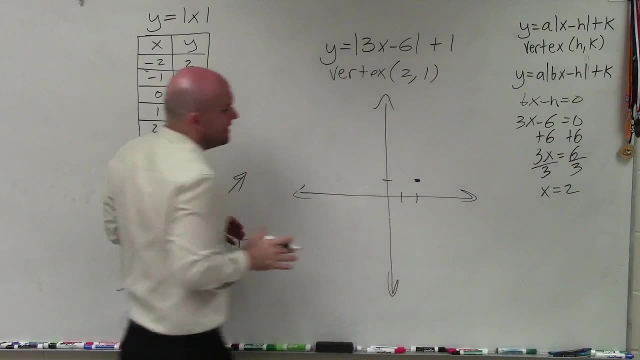 up one unit Now. the next thing I want to do is I need to be able to identify what exactly is my graph going to look like, And I can't take this graph and just plug it in there, because this b is what the b is going to be doing, That's going to now vertically stretch. 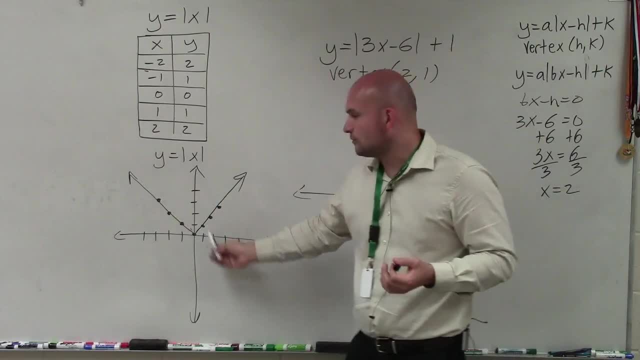 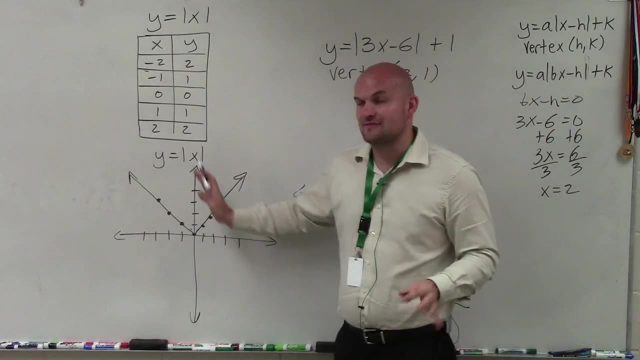 my graph. So this simple over 1, up 1, over 2, up 2 is not going to apply. So the easiest way to be able to identify what are the other points in the graph is to either graph two points to the left or graph two points to the right and then use my axis of symmetry. 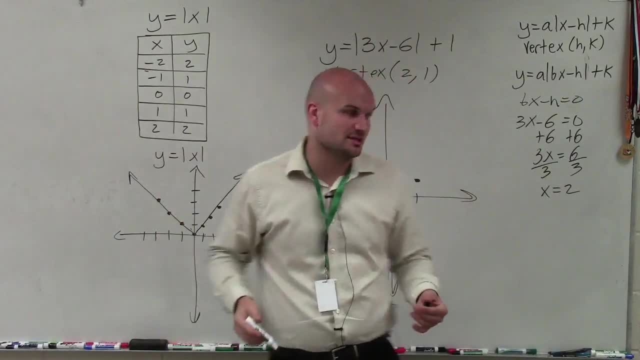 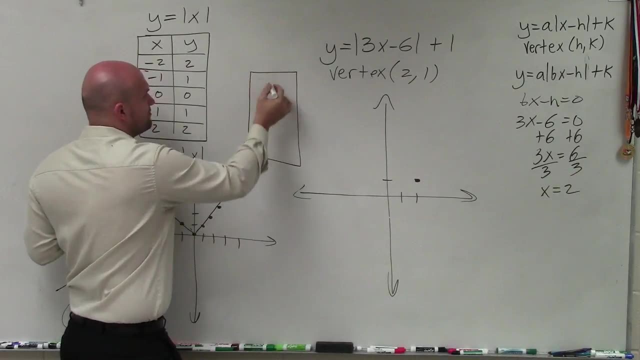 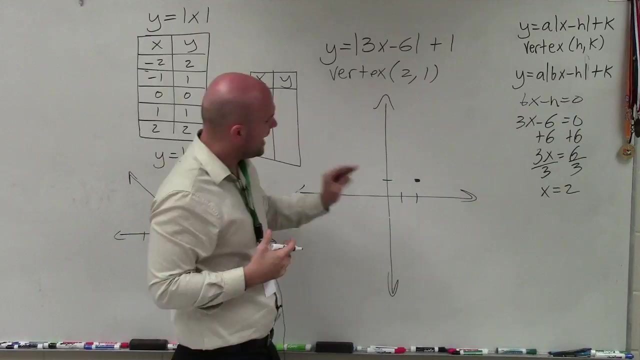 which goes to my vertex To reflect, to find the other two points of the graph, So to find at least any two points in the graph. we kind of need to identify: well, which points do I need to pick to the left or to the right? And really you can pick any points you want to. I think it's. 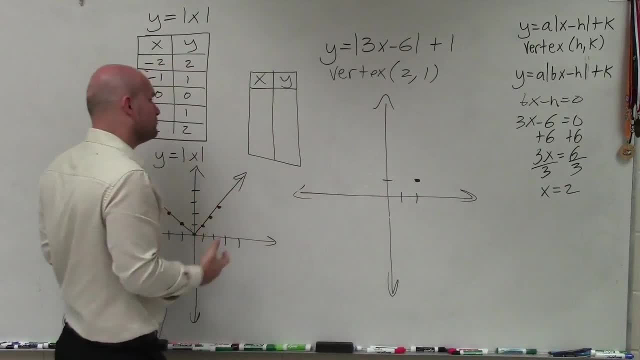 always easier to pick numbers that are going to be simple. So if I pick two points to the left, I have 1 and 0. I would like to plug 1 and 0 into my equation. I think that would provide some very basic information. 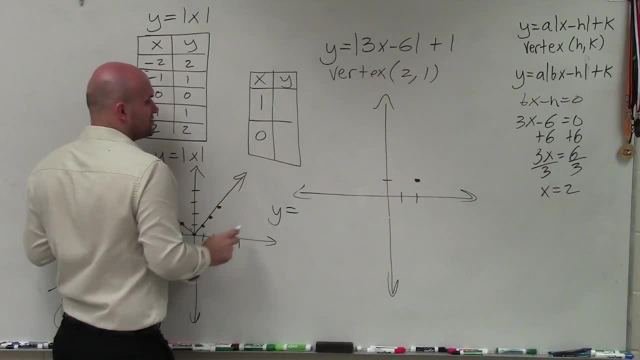 But I'm going to do three basic operations. So to find the 1, if I know the x value is 1, what is going to be the y value? So I plug 1 in for x. So I have 3 times 1, minus 6,. 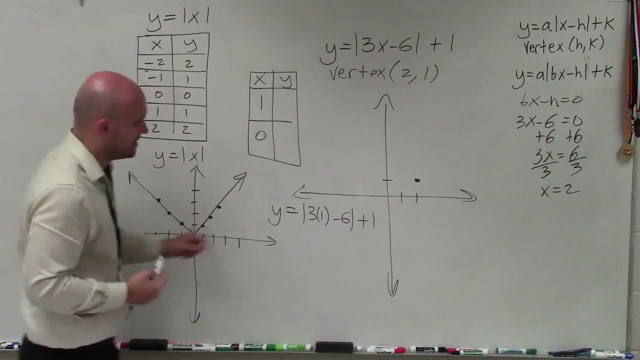 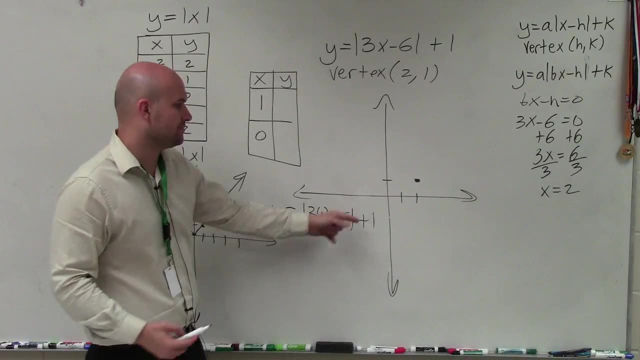 plus 1.. Now I'm going to kind of do this in my head, but I'll say it out loud: 3 times 1 is 3.. 3 minus 6 is negative, 3.. Absolute value of negative 3 is positive 3.. 3 plus. 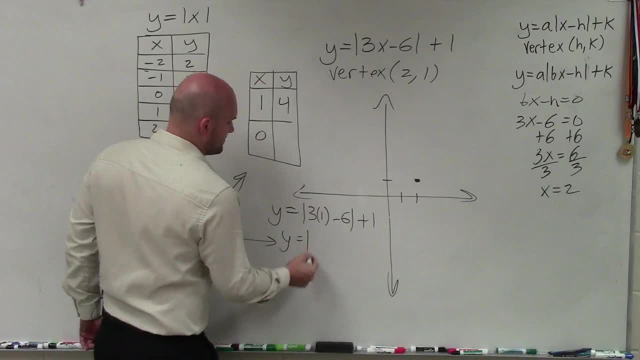 1 is 4.. And then at 0,. I'll do that for the same thing 3 times 0 is 0.. I'm going to plug in 3.. I'm going to plug in 2.. 3 minus 4 is negative 3.. Excellent, Perfect, All right. 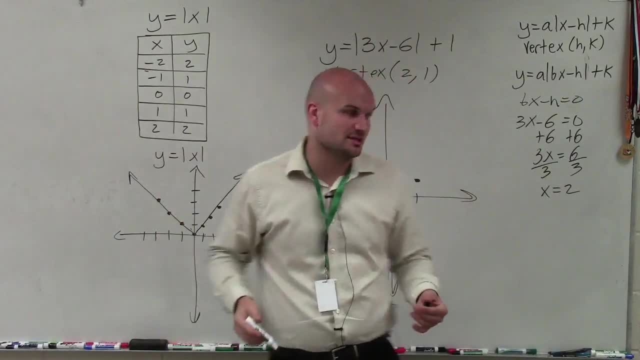 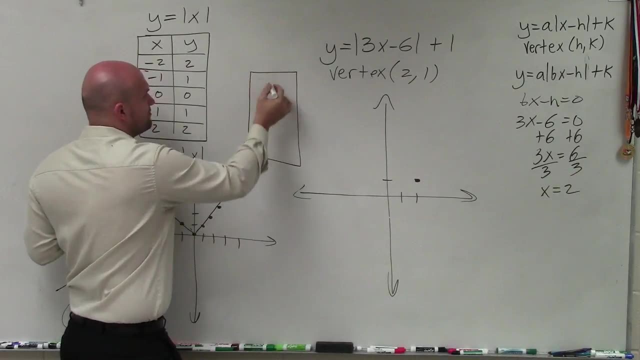 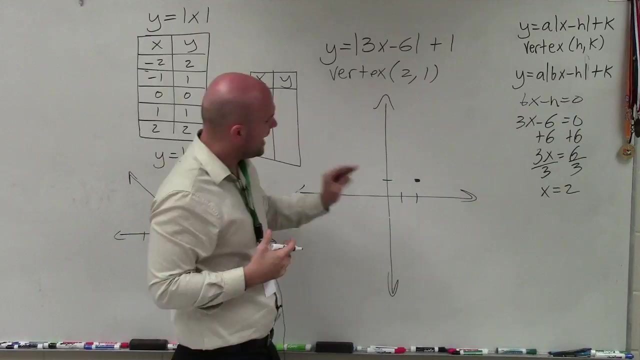 which goes to my vertex To reflect, to find the other two points of the graph, So to find at least any two points in the graph. we kind of need to identify: well, which points do I need to pick to the left or to the right? And really you can pick any points you want to. I think it's. 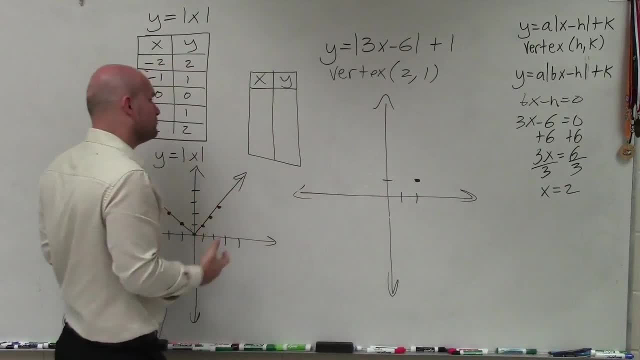 always easier to pick numbers that are going to be simple. So if I pick two points to the left, I have 1 and 0. I would like to plug 1 and 0 into my equation. I think that would provide some very basic information. 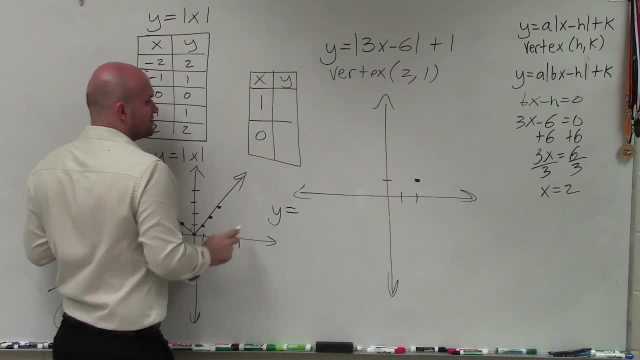 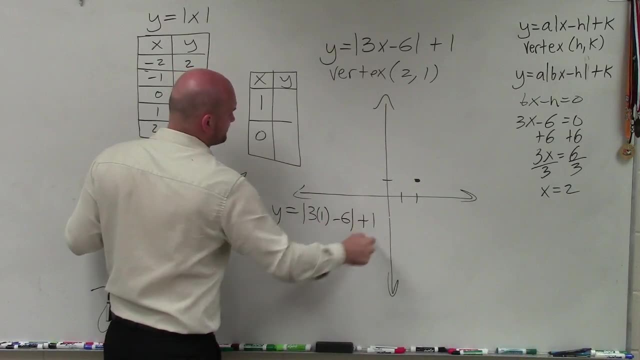 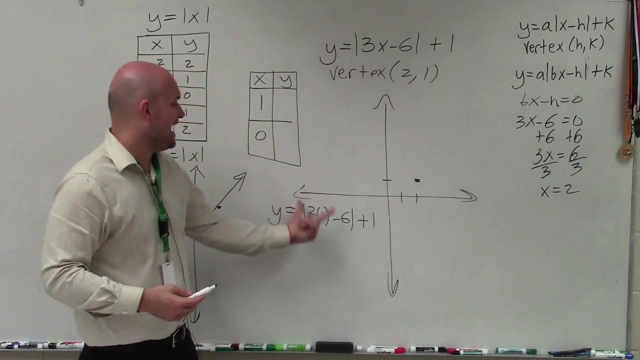 ANDY 블�litzenfeld, PhD, MPH, H~ Questions No. All right, OK, Let's imagine if Iелаived at 0.. So as the higher the sin is, or b, all, the also more of these values start indicate that. 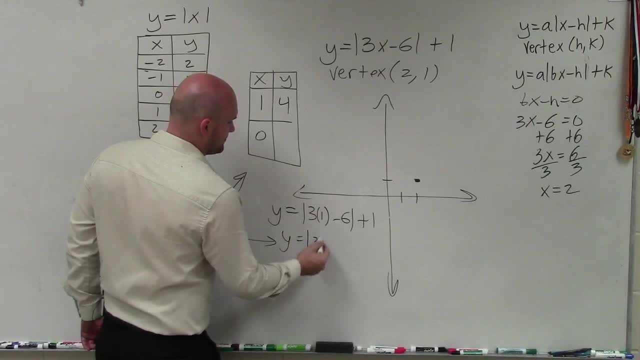 squared times 0.. One of these values is 7.. The first one lets me create the indexing. What does this do? When you sum things up to it, we use the negative generalization And then let me represent all those values. So I plug 1 into for x. 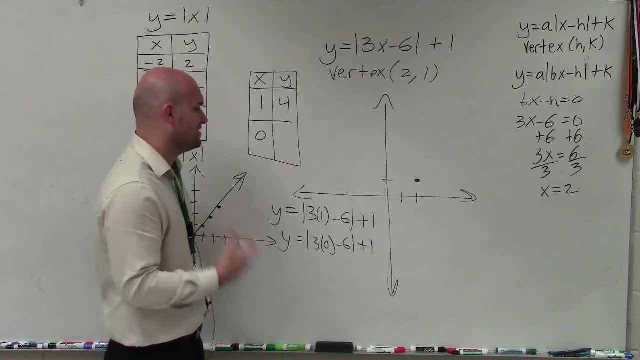 So I have 3x plus 1 minus 6 plus 1, and then at 0. I will do this in my head, but I'll say it out loud Three times: one is three minus 6 is negative, 6.. Absolute value of negative 6 is positive, 6.. Positive 6 plus 1 is 7.. So that 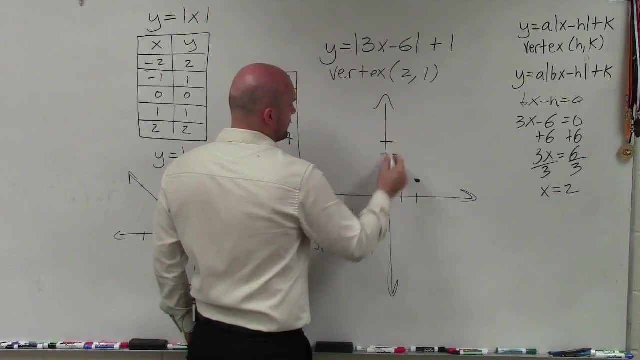 means I go over 1.. Now I got to go up 4.. 1,, 2,, 3,, 4.. And then I have to go up 7.. 1,, 2,, 3,, 4,, 5,, 6, 7.. 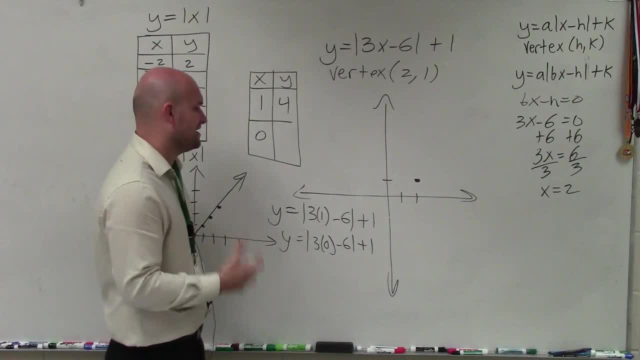 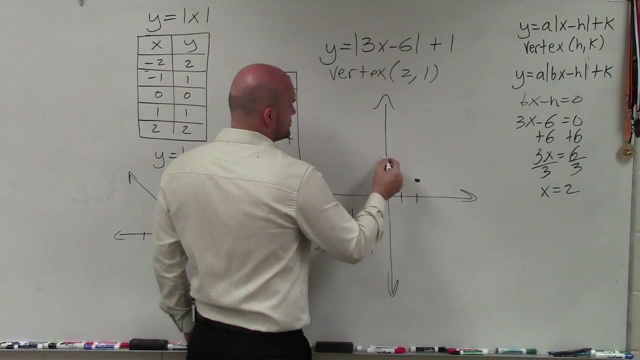 times 0 is 0.. Minus 6 is negative 6.. Absolute value of negative 6 is positive 6.. Positive 6 plus 1 is 7.. So that means I go over 1.. Now I've got to go up 4,, 1,, 2,, 3,, 4.. 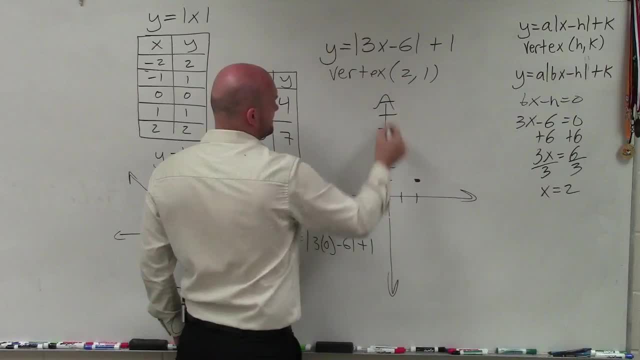 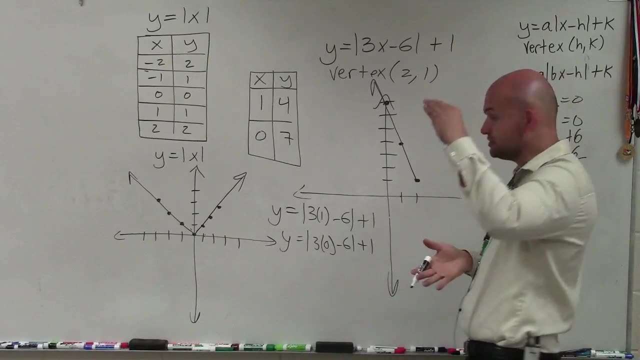 And then I have to go up 7,, 1,, 2,, 3,, 4,, 5,, 6,, 7.. So you can see that my graph, compared to my paragraph, is much steeper. It's been vertically stretched.